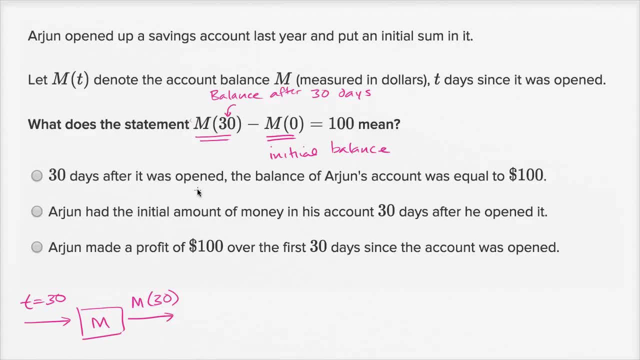 are consistent with that: 30 days after it was opened, the balance of Arjun's account was equal to 100.. No, that's not what that's saying This statement right over here, that the balance 30 days after opening this statement right over here. 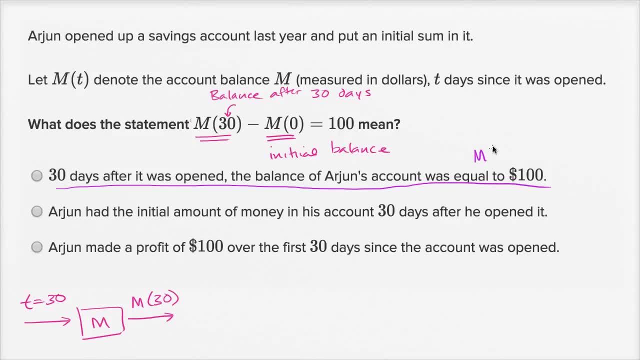 this would be equivalent. this is equivalent to saying that M of t of 30, this is the balance 30 days after it was opened- is equal to 100.. That's not what they tell us here. They tell us that the difference 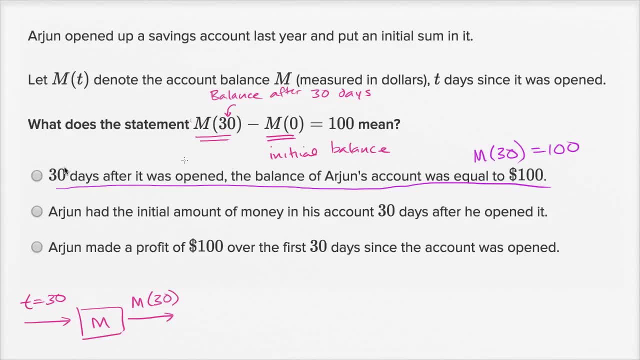 between the balance after 30 days and the initial balance of that is 100.. So we can rule that one out. Arjun had the initial amount of money in his account 30 days after he opened it. So if he had the same amount, 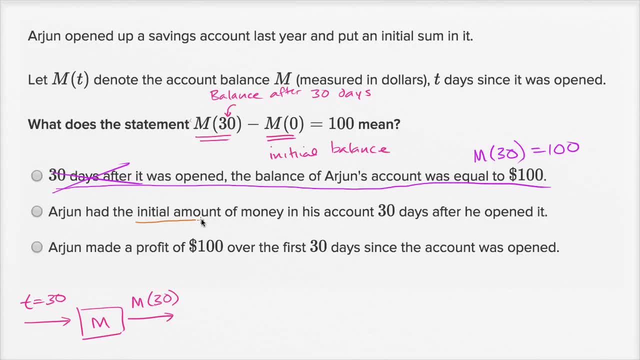 if he had the initial amount. let me write this down: So had the initial amount of money. the initial amount of money is M of zero. So they're saying he had the initial amount of money in his account 30 days after he opened it. 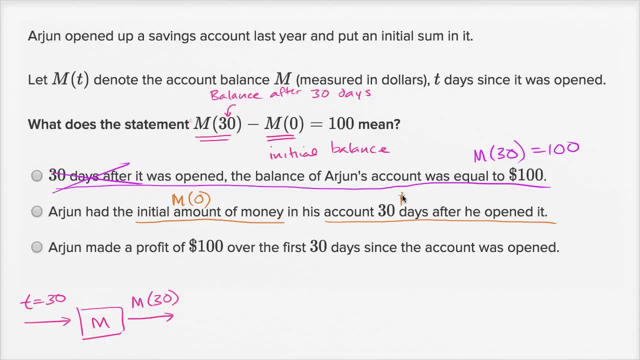 Well, the amount that he has in his account 30 days after he opened it is M of 30. So if these are the same amounts of money, then this, in order to be consistent with this, you would have had an equation like this: 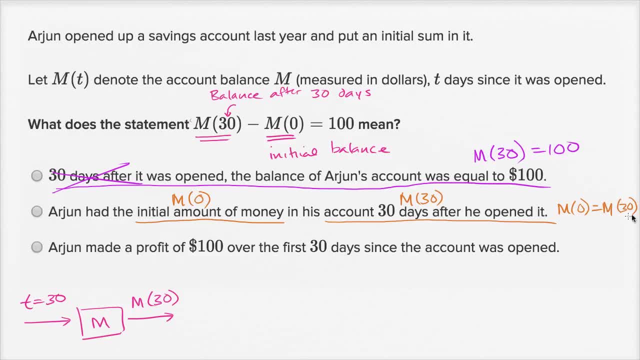 M of zero. the initial amount is equal to the amount after 30 days. That's not what they told us over here, So we can rule that out. And then, finally, we have the choice. Arjun made a profit of $100,. 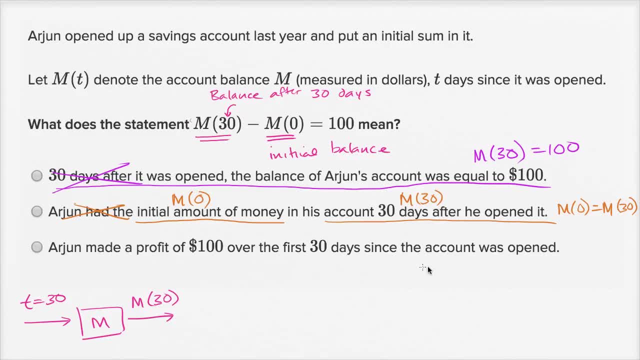 Arjun made a profit of $100, over the first 30 days since the account was opened And that seems reasonable that his balance is $100 higher. The difference between: if you take his initial balance and subtract it from his balance after 30 days. 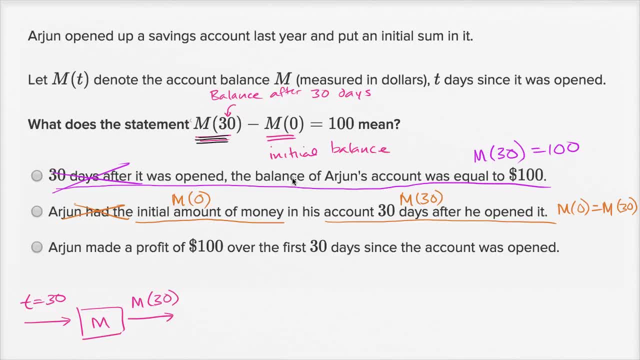 it's 100, that this right over here is 100 higher than his initial balance. So it makes sense that maybe he got that profit out of notes and interest or something else that he got in his bank account over the first 30 days.